drive through the total area, Because the amount of energy that's needed to do this, or the amount of energy that's needed to do this, is going to be t-threaded. But we want to save the time. We don't want to, we don't want to drive through with all of this and we're not going to let anything that's inside all of this. So we're going to. 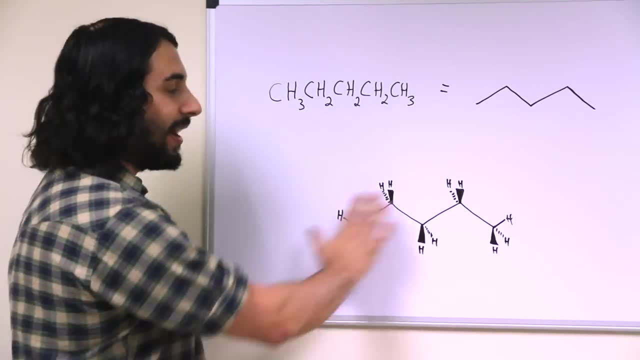 want to save the time. we don't want to. we don't want to draw all these hydrogen, so we're not going to draw them. this is what we're going to draw, but this is what that really means, and if you haven't seen this kind of notation, 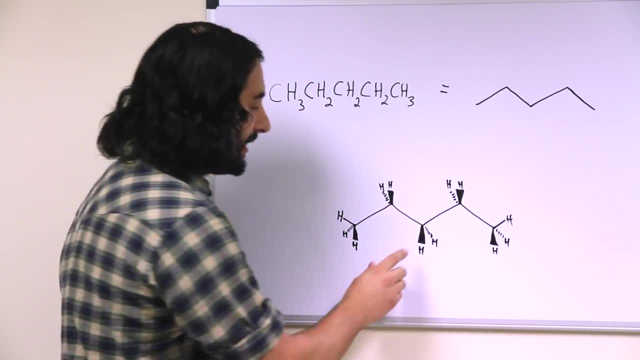 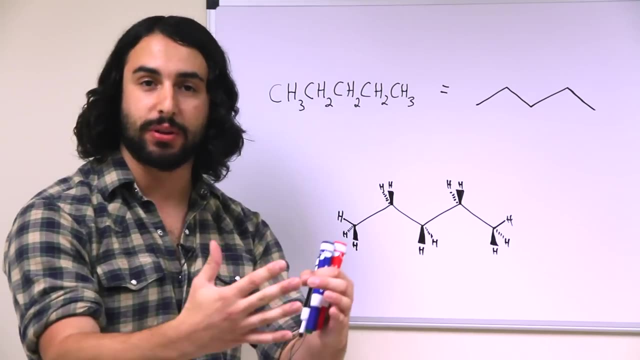 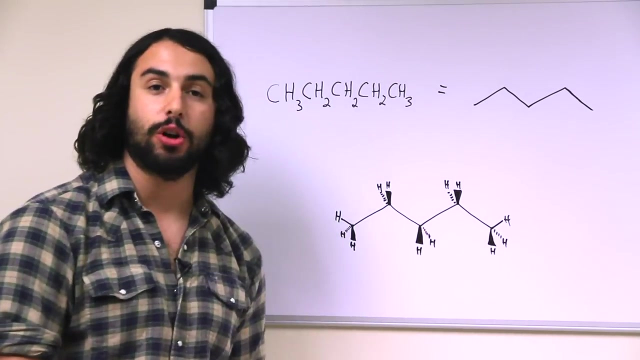 yet, with the dash and the wedge lines, what this means. each wedge bond implies that that atom is coming towards you. it is coming out of the plane, of the board, of the page, so this hydrogen is extended this way, and the dash bonds are going into the page or into the board, so this hydrogen is further away from you than 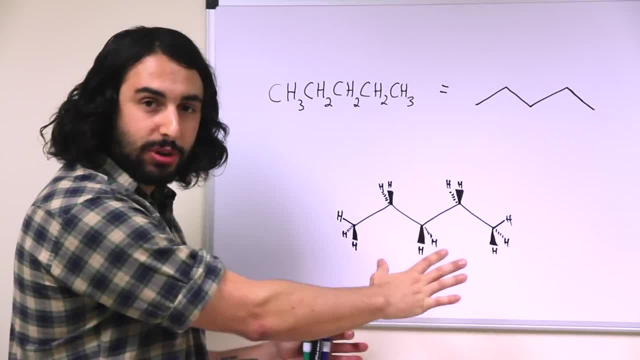 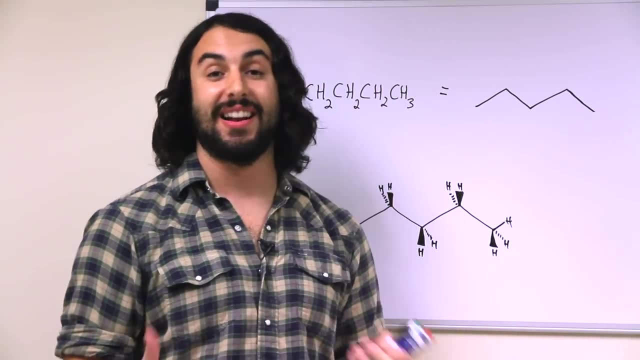 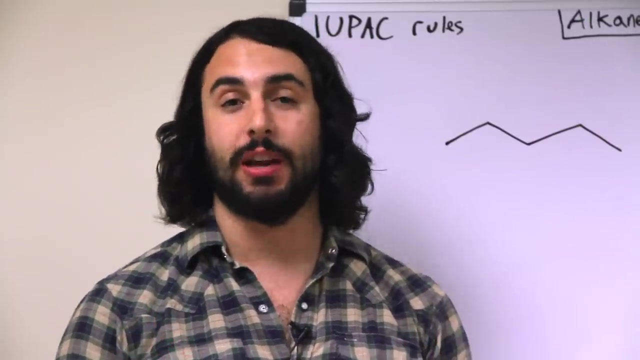 the plane of the board, and so that obeys tetrahedral geometry, we can see that all of the atoms are accounted for, and this is the kind of notation we are going to use from now on as we learn organic chemistry. so, as chemists, we're gonna want to be able to communicate with each other. 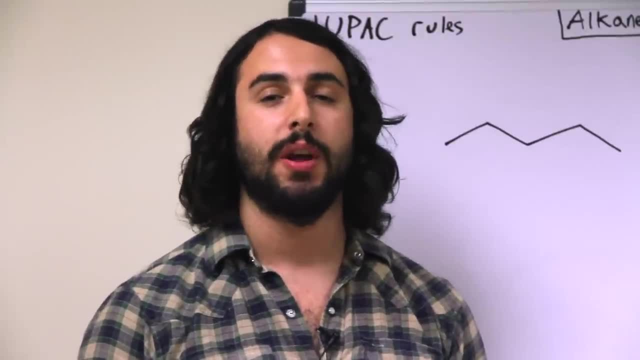 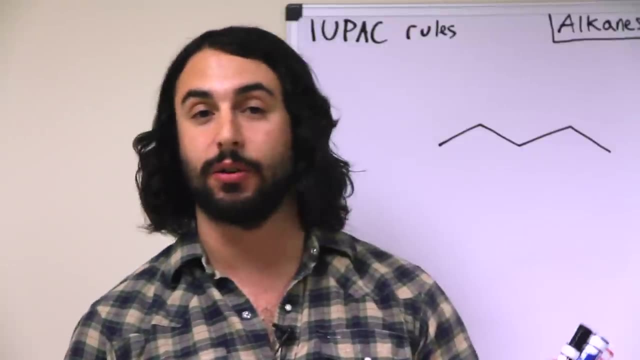 efficiently. this means that when we want to discuss a particular molecule, it may be easier to refer to it by name, but that name is going to have to be of a type that every scientist, wherever they are in the world, is going to agree about what molecule we're talking about. so 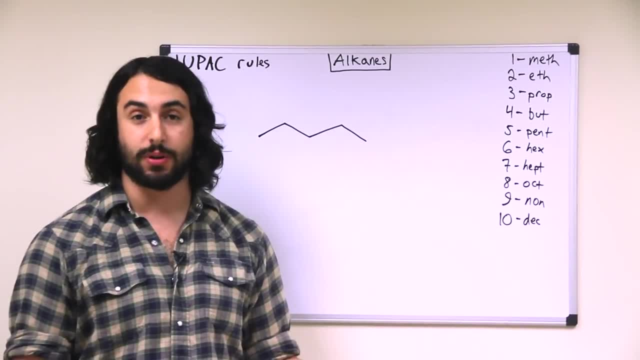 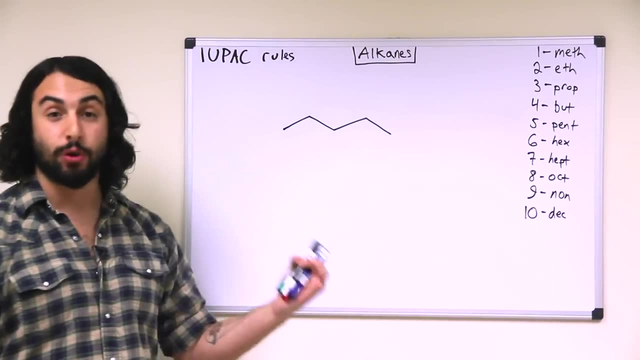 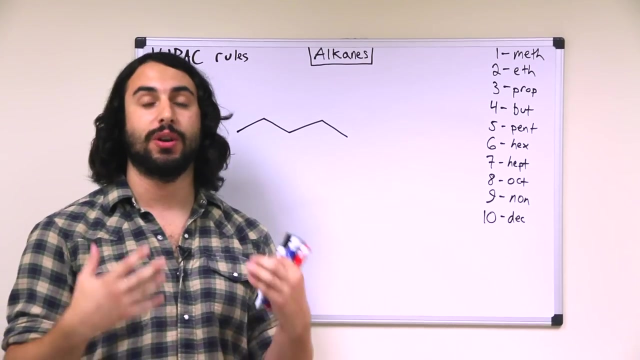 we're gonna have to learn a set of rules that are completely arbitrary, but if we all follow them, we will all be able to name molecules the same way. so an organization called IUPAC- this is the International Union of Pure and Applied Chemistry- has come up with these rules that we can follow to assign names to. 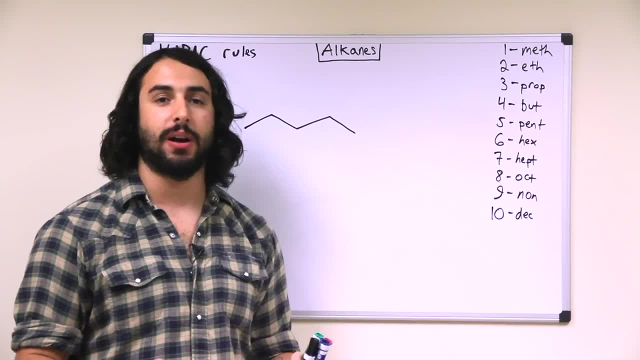 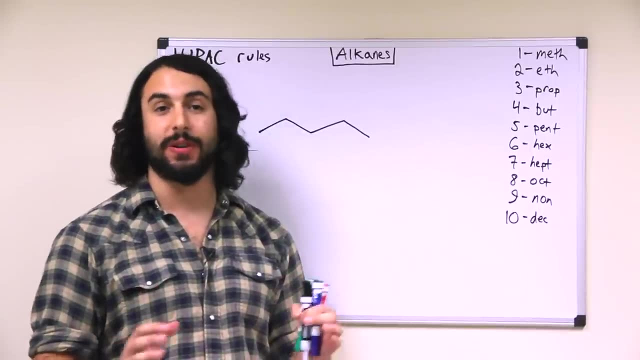 any organic molecule. so the first kind of molecule that we want to talk about is alkanes. so alkanes are a type of hydrocarbon, a hydrocarbon being a molecule consisting only of carbon and hydrogen, and alkanes are hydrocarbons that are fully saturated. this means that they contain 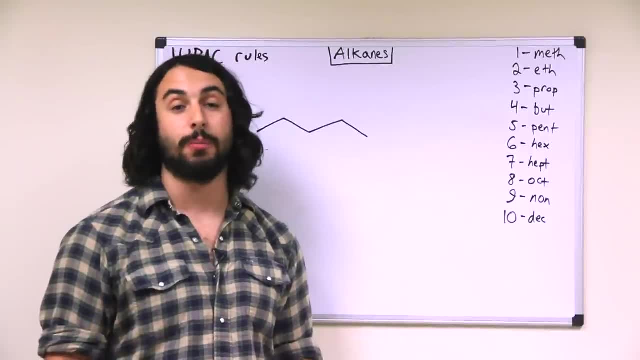 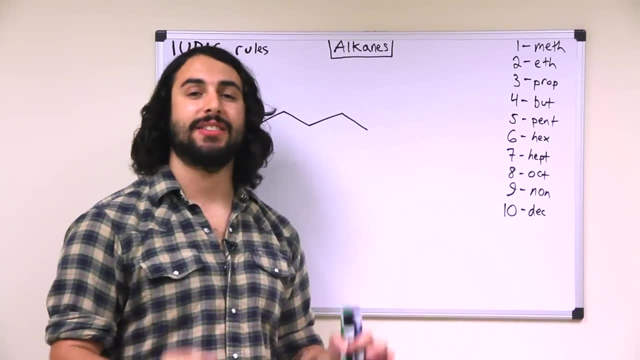 the maximum number of hydrogen is possible. in other words, no double or triple carbon-carbon bonds. we have only single carbon-carbon bonds. so any alkane is going to bear the suffix "-ane", so that is the suffix that will be present in the molecule. 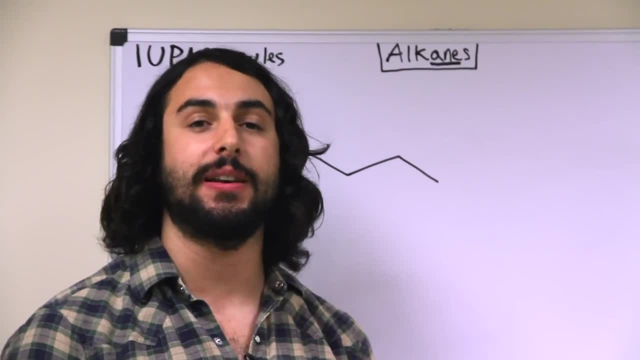 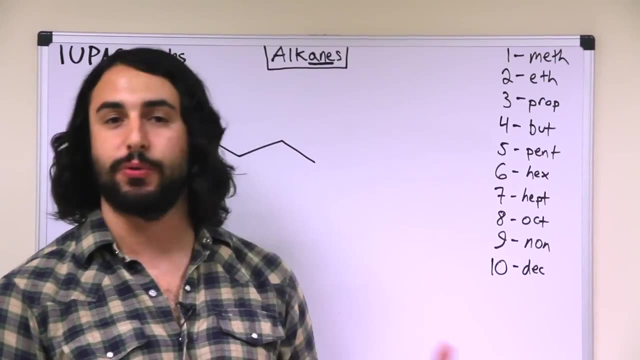 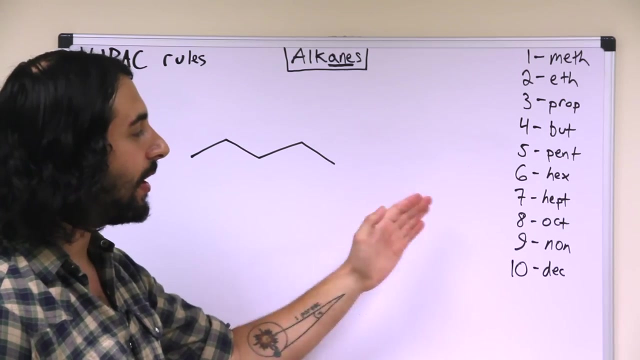 the prefix is going to be determined by how many carbons are in the molecule. so depending on what your particular chemistry class is like, you may have to memorize more or fewer prefixes, but the very least we're all gonna have to know these ten. so meth, eth, prop, but pent, hex, hept, oct, non dec. these would be the 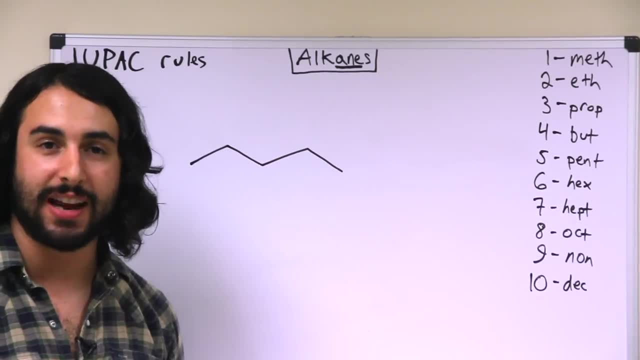 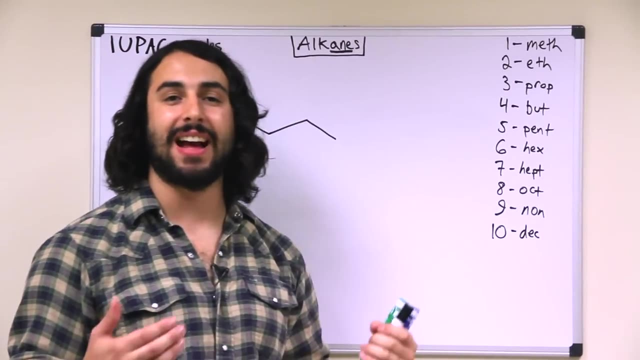 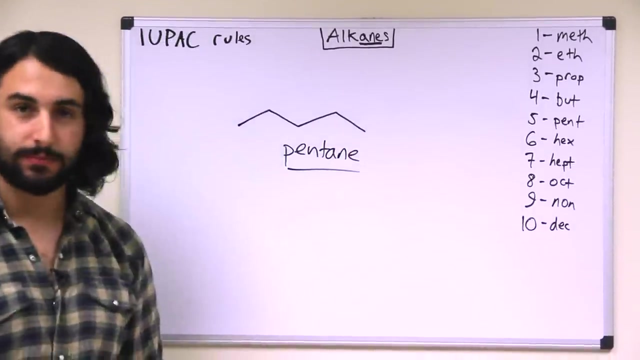 prefixes of a given molecule. so let's take our five carbon alkane that we were looking at before right: one, two, three, four, five. that is going to be pent for hex and it is an alkane, so "-ane" that makes this molecule pentane. so while it 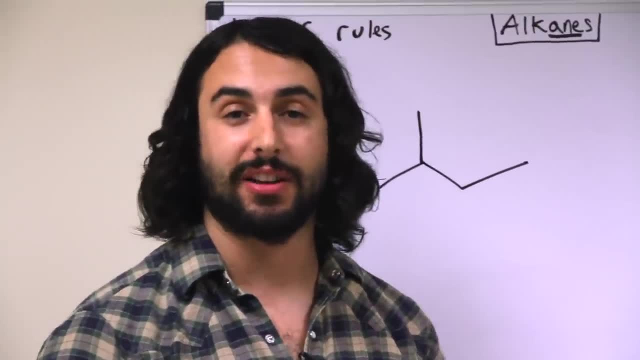 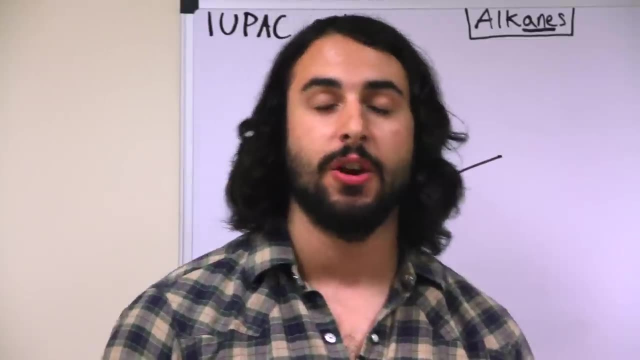 would be wonderful if every molecule we had to name were as simple as a straight chain alkane. that's not going to be the case. molecules have a variety of substituents, which are smaller groups branching off of a main chain. so let's look first at a very easy example of a branched chain. 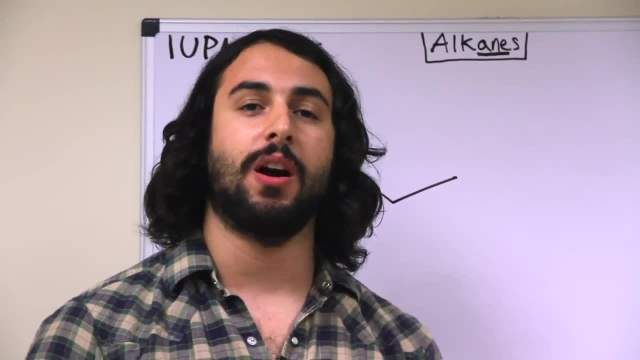 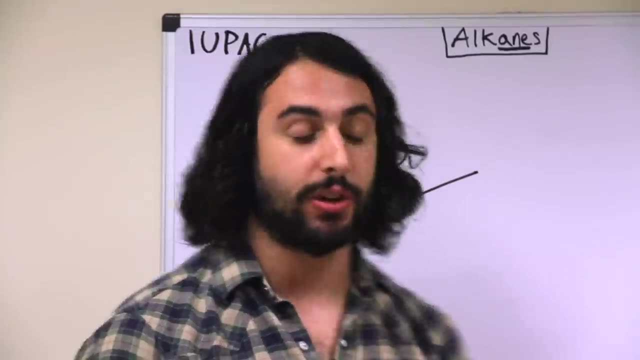 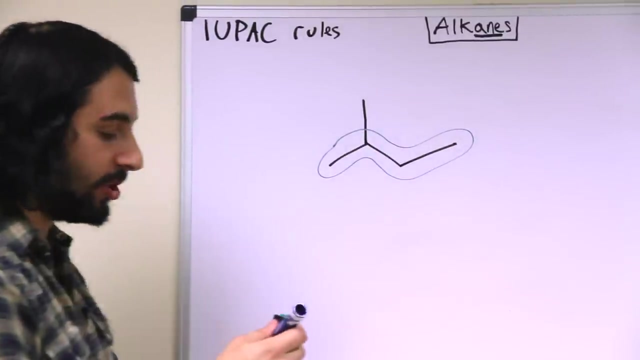 alkane. so what we need to do when we are naming a hydrocarbon is we need to identify the longest chain of carbons in the molecule. so right now that's going to be pretty simple. we can see that there is a four carbon chain here and 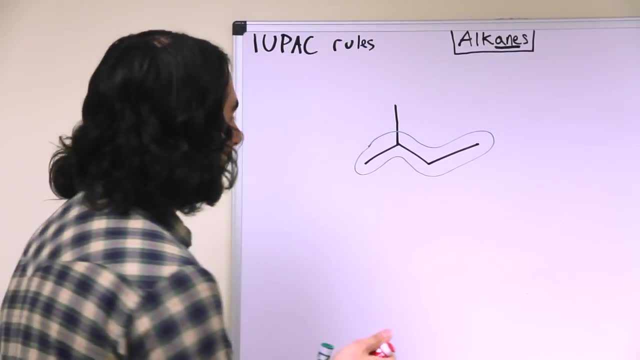 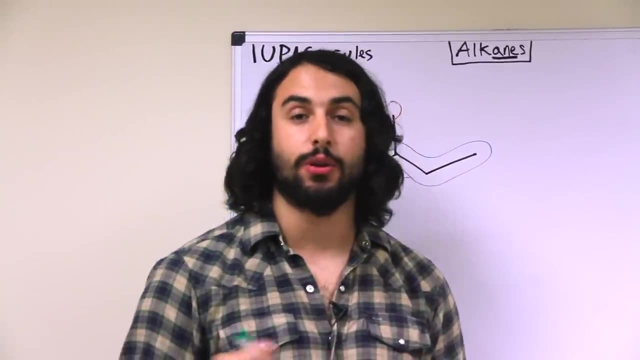 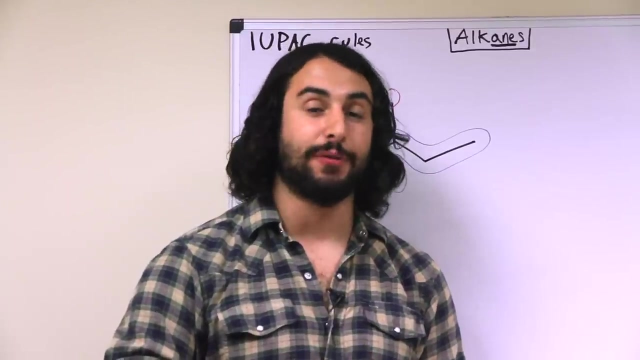 there is a one carbon substituent branching from the main chain. so now that we have identified the longest chain in the molecule, we're going to have to number it. now there are two options. you can go left to right, or we are going to choose the direction that gives the substituent occurring. 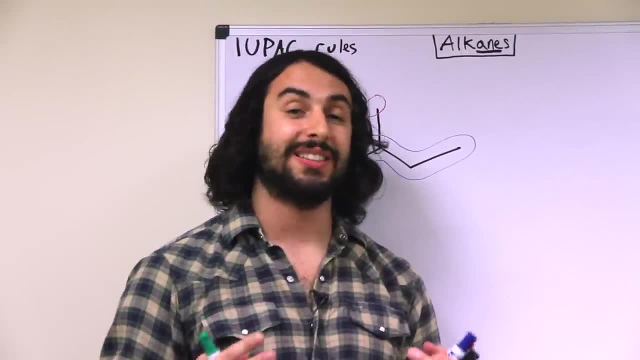 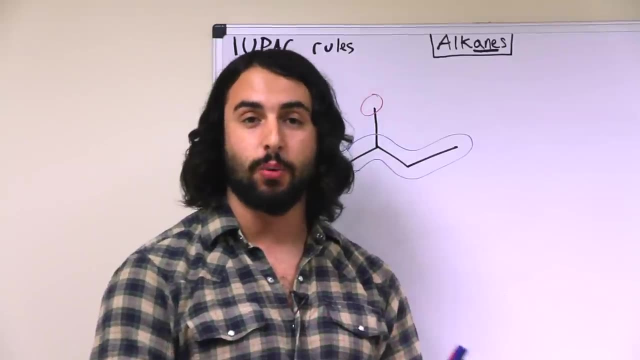 sooner, or on the lower numbered carbon. once again, this is a completely arbitrary rule. it has nothing to do with nature. but if we all agree that these are the rules we're going to follow, we will all be able to assign the same name, same name, to the molecule. so here we are, going to number the molecule left to. 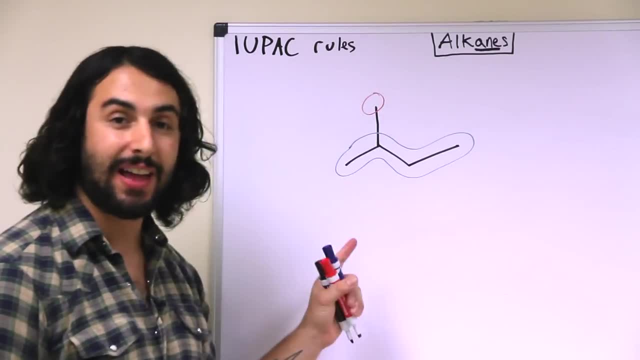 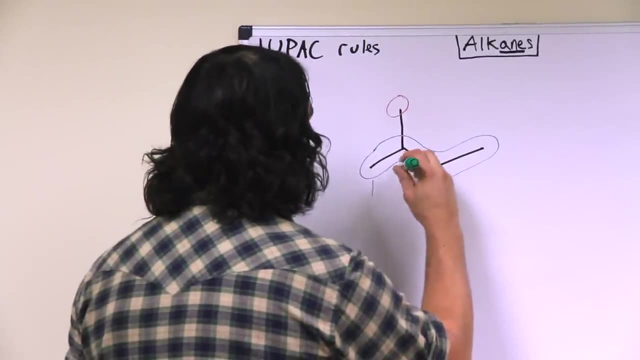 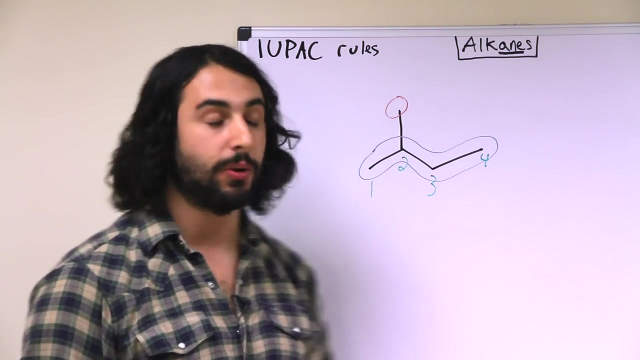 right and not right to left, because if we number from the left, the one carbon substituent will occur sooner. so this is going to be 1, 2, 3, 4, like that, and the one carbon substituent is going to be on carbon 2. if we had numbered from this direction, it would